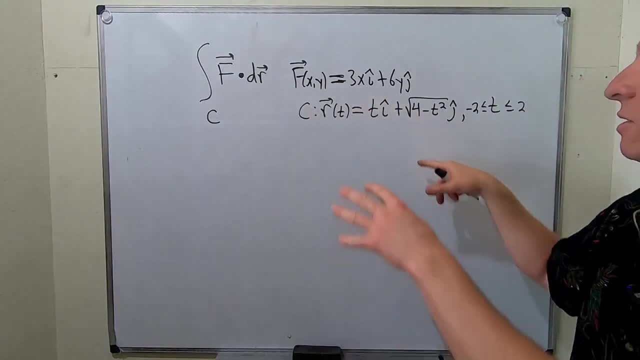 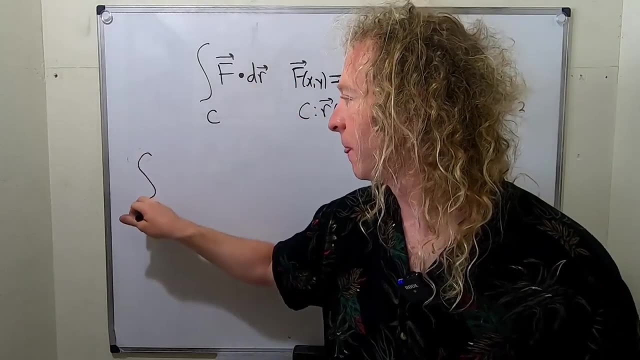 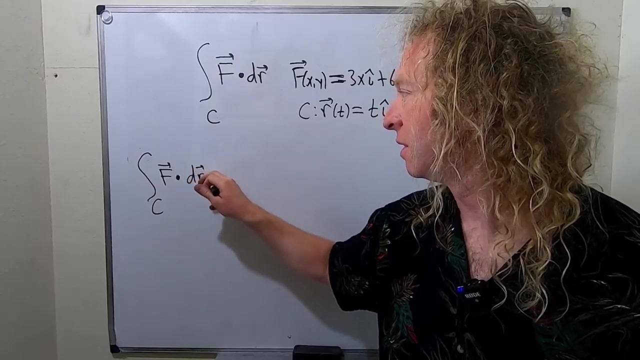 this means? So this is a vector field and this here is a curve, and it's given by this vector valued function from negative two to two. So this thing here, so this line, integral f dot- yeah, that's a dot- product dr is equal to the following: So we're going to go from a to b. 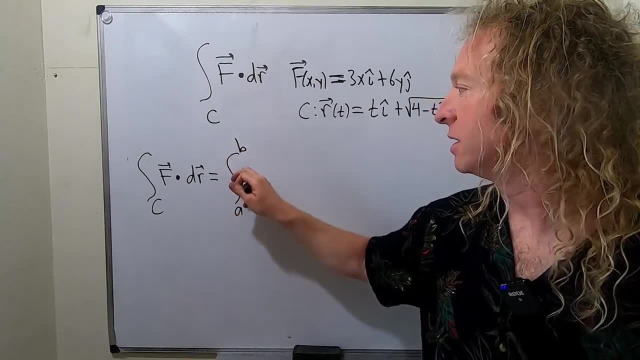 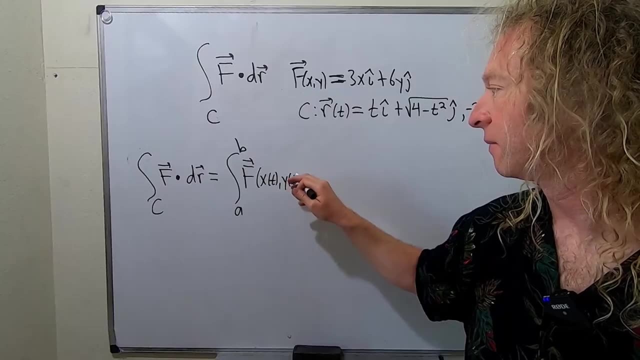 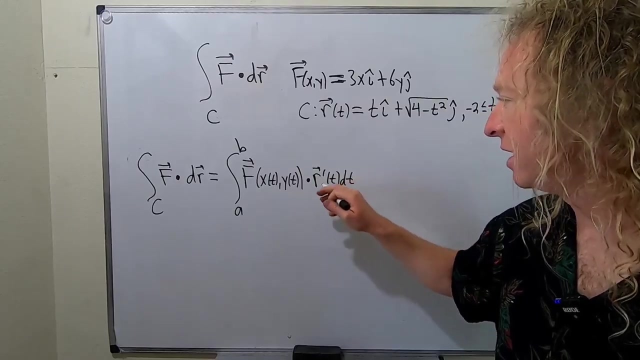 so I'll just write a and b for now. so a to b. and it's f of x of t, comma y of t, dotted with the derivative of r, dt, And again, that is a dot product. Okay, so what does this mean essentially? So we're going to go from a to b, so I'll just write a and b for now. so a to b. 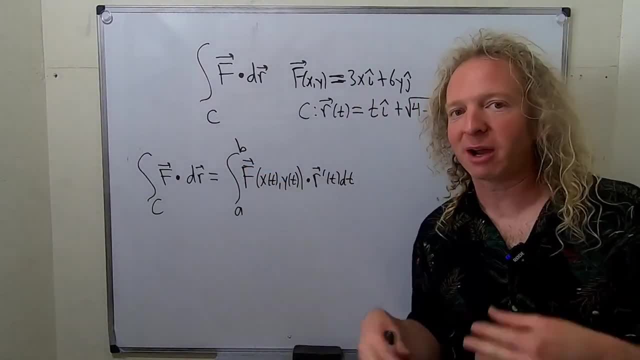 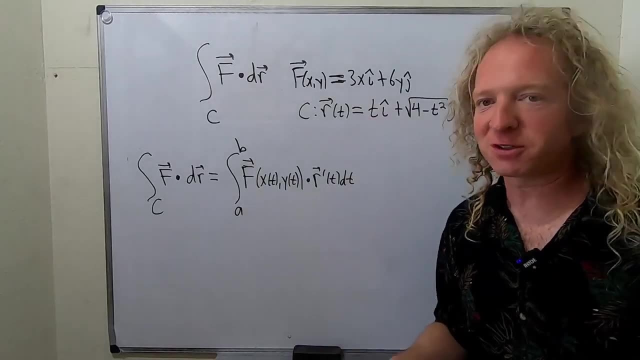 dotted with the derivative of r, dt, And again, that is a dot product. Okay. so what does this mean And what is going on? So one way to think about how this works is if f was a force field. so in physics you have these things called force fields. So if f is a force field, okay. 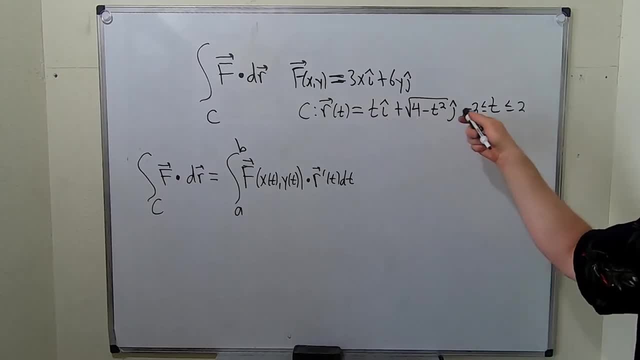 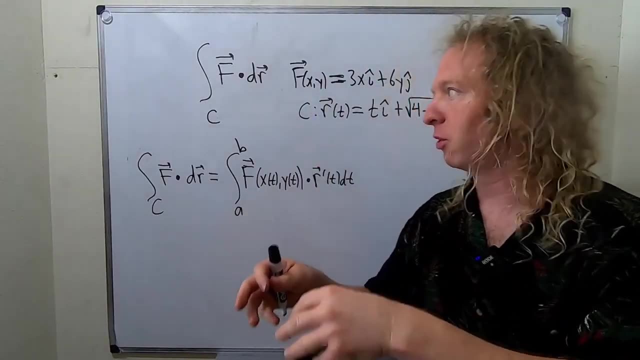 and then you have a particle moving along this path from negative two to two, then this line integral will give you the work done to move that particle from negative two to two. So the line integral gives you the work. okay, that's one way to look. 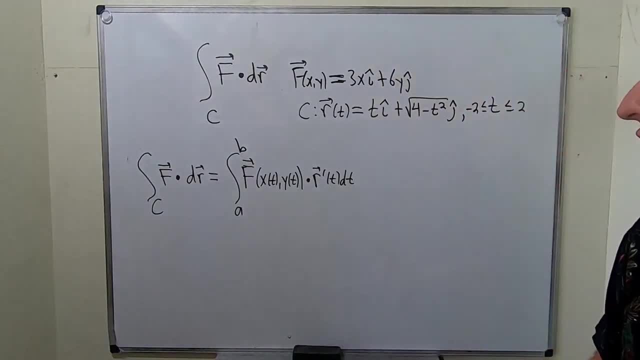 at it. In this problem, though, we're mainly concerned with the computation. so this is the definition, this is the formula, So now we just have to figure out what everything is here. So we already have r, we already have x and y. let's go ahead and specify them. to be more, 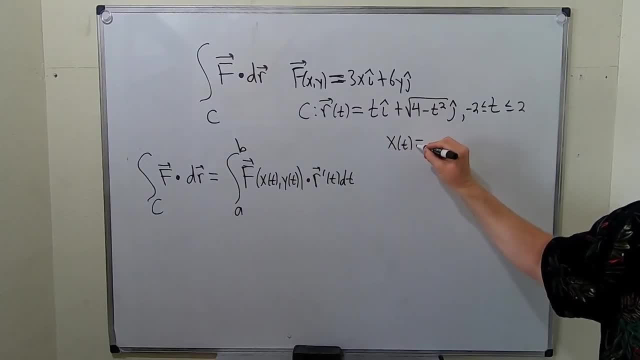 clear. So x of t in this problem is equal to t and y of t is equal to this here. I'm going to leave it like that for now. so 4 minus t squared, And we do have to take the derivative. so that's. 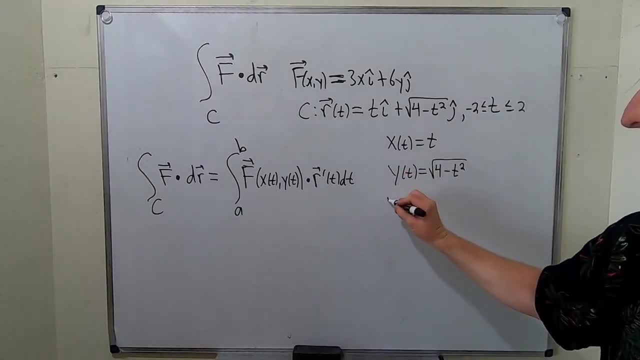 what I was thinking like: oh, I want to rewrite it because I want to differentiate it, So let's go ahead and rewrite it now, Because we do have to differentiate it at some point. Okay, so we're going to take these and we're going to plug them into our 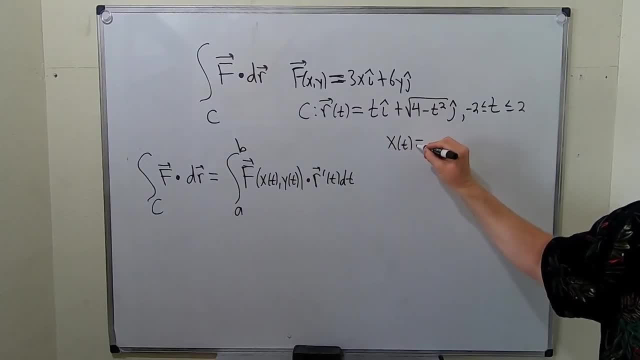 clear. So x of t in this problem is equal to t and y of t is equal to this here. I'm going to leave it like that for now. so 4 minus t squared, And we do have to take the derivative. so that's. 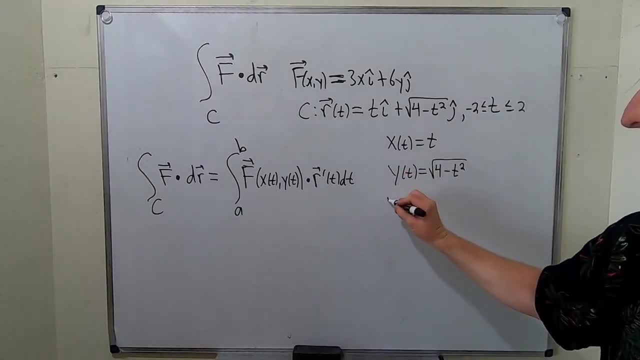 what I was thinking like: oh, I want to rewrite it because I want to differentiate it, So let's go ahead and rewrite it now, Because we do have to differentiate it at some point. Okay, so we're going to take these and we're going to plug them into our 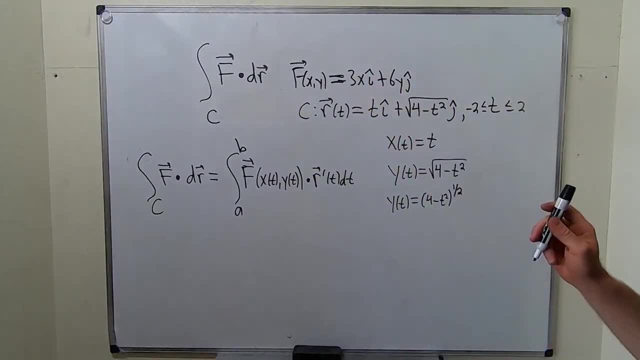 vector field and then we have to compute our prime. So, in order to compute our prime, we need the derivatives. So let's do that. I think I could squeeze it in here. So x prime of t is simply one, because the derivative of t is one. To compute y prime. I'm going to look. I'm going to look here. 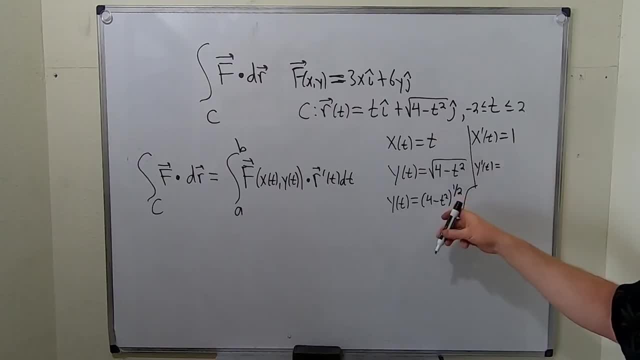 So y prime of t is one, and then I'm going to look here. So y prime of t is one and then I'm going to prove y prime of t. So we have to use the chain rule. You treat this piece as the inside piece. you put the 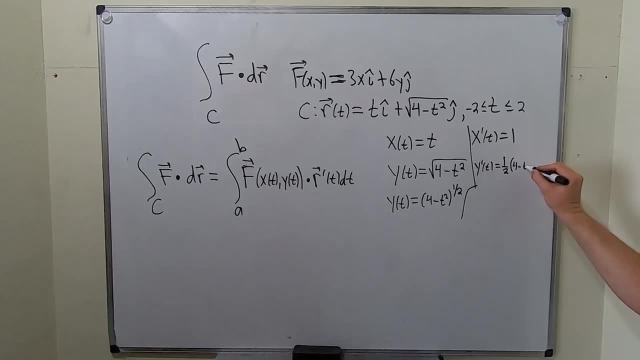 one-half in the front. so we get four minus t squared. One-half minus one is negative one-half times the derivative of the inside. so negative two t. It might be kind of hard to see. hopefully not So. y prime of t. 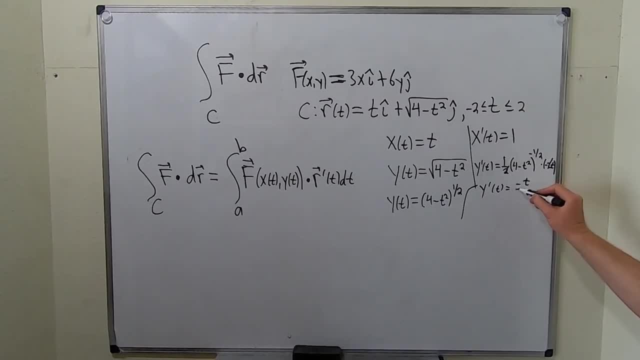 the twos cancel. so we get negative t, and I'm going to bring this bad boy downstairs. Square root four minus t, squared to the one-half. when you bring it down, it becomes positive. okay, so we have our x prime. we have our y prime now. 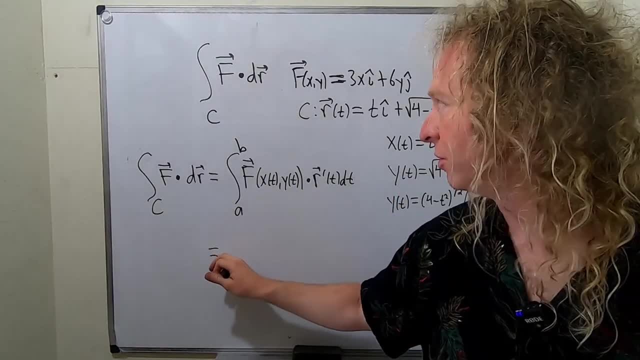 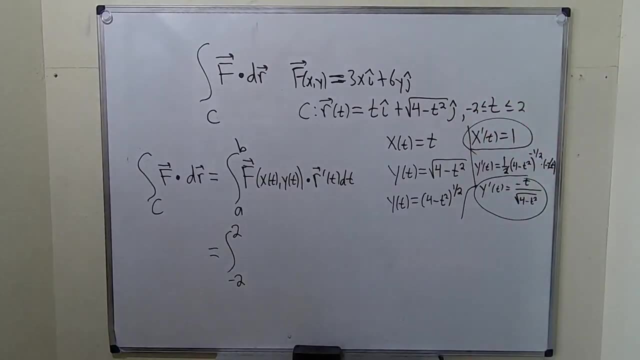 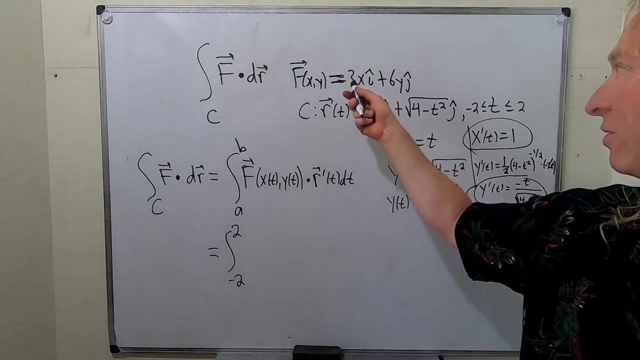 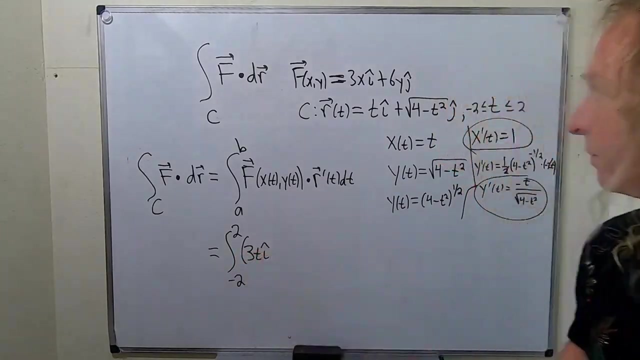 let's go ahead and keep working here. so this is equal to: so we're going from negative 2 to 2, negative 2 to 2 and f is this. so we're going to plug in our x and y into this. it's really ridiculous looking. so it'll be 3t i-hat. so I'm going to go slow: 3 t i-hat plus 6. 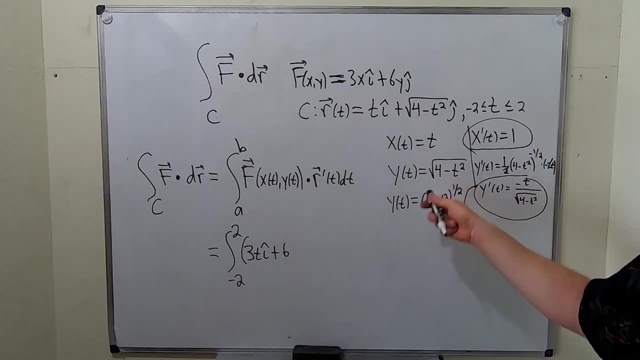 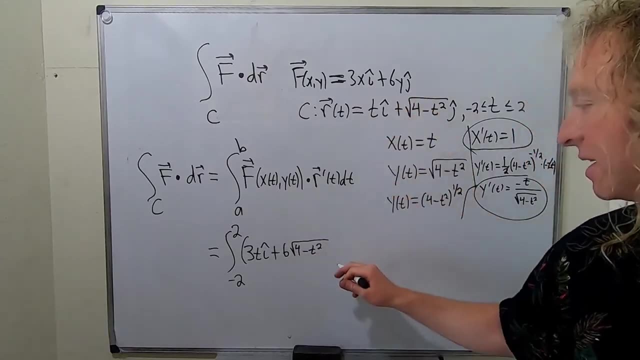 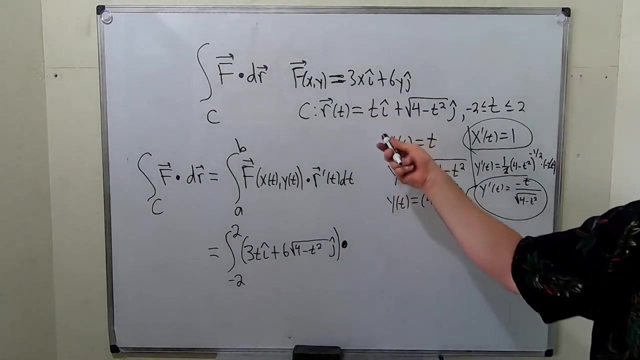 and then what was y? well, y is this. I'm going to leave it like this. I'm going to leave it as a square root, square root four minus t, squared, and then we have our j hat. let's not forget that parentheses dot, right dot, and then the derivative of this, so we can. 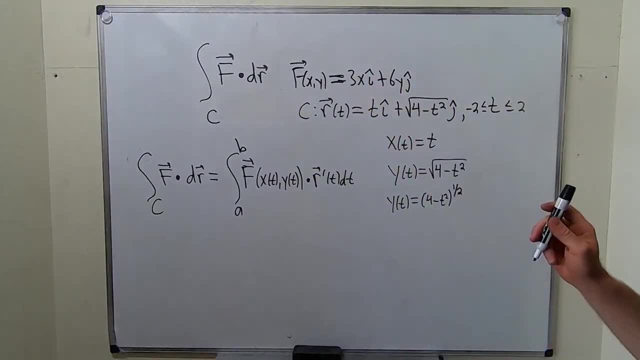 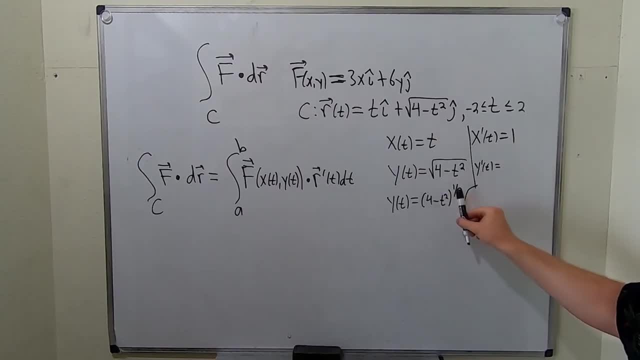 So we have to use the chain rule. You treat this piece as the inside piece. you put the one half in the front, so we get four minus t squared. one half minus one is negative one half times the derivative of the inside. so negative two t Might be kind of hard to see. hopefully not So y prime of t. 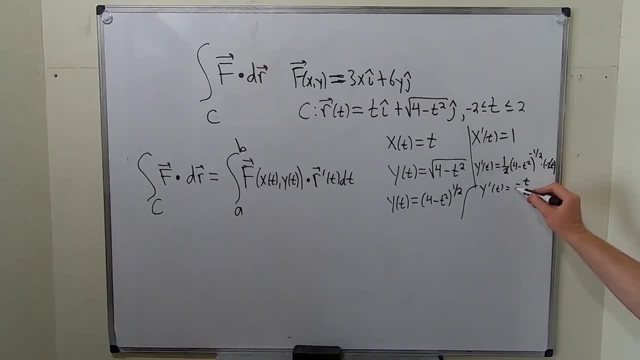 the two's cancel. so we get negative t, and I'm going to bring this bad boy downstairs. square root four minus t, squared to to the one half, when you bring it down, it becomes positive. okay, so we have our x prime. we have our y prime now. 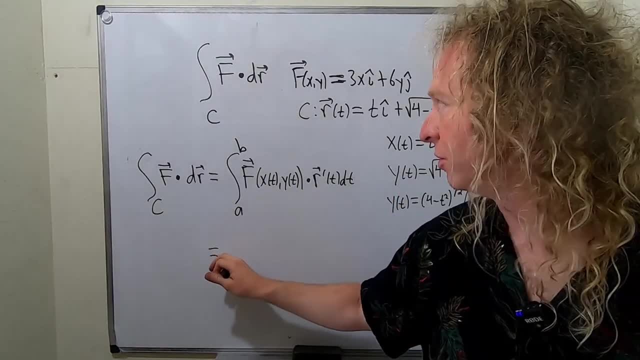 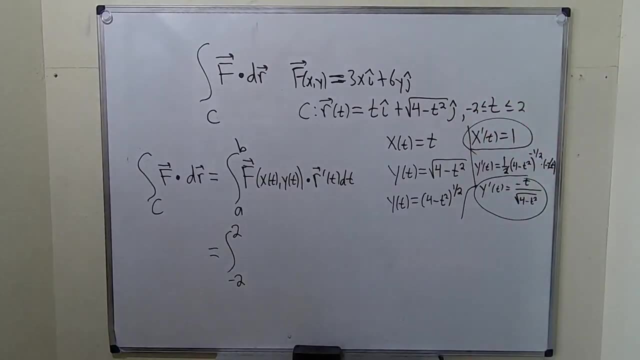 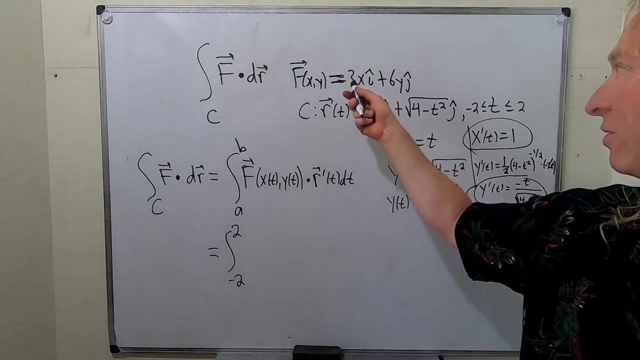 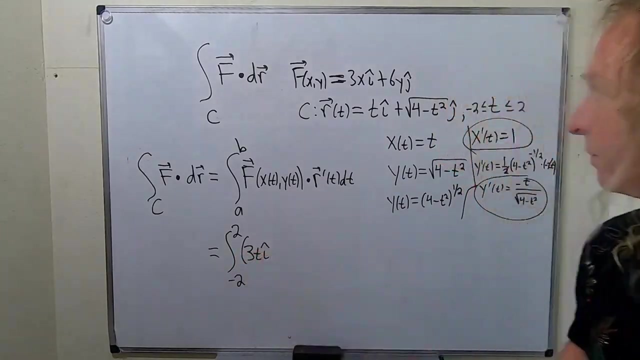 let's go ahead and keep working here. so this is equal to: so we're going from negative 2 to 2, negative 2 to 2 and f is this. so we're going to plug in our x and y into this. it's really ridiculous looking. so it'll be: three t i hat. so i'm gonna go slow. three t i hat, plus six. 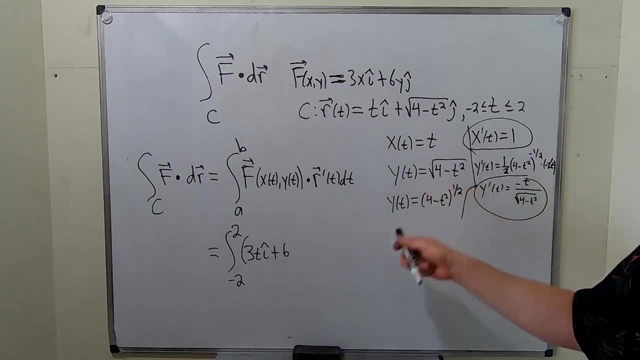 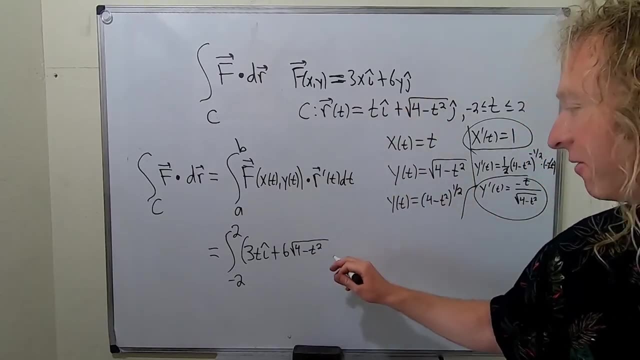 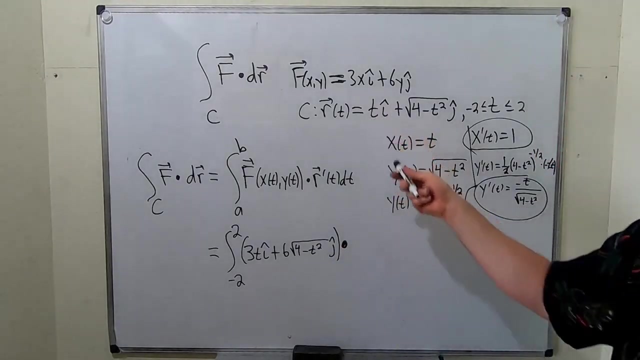 and then what was? y? well, why is this? I'm going to leave it like this. I'm going to leave it as a square root, square root 4 minus t, squared, and then we have our J hat. let's not forget that parentheses dot, right dot, and then the derivative of this, so we can. 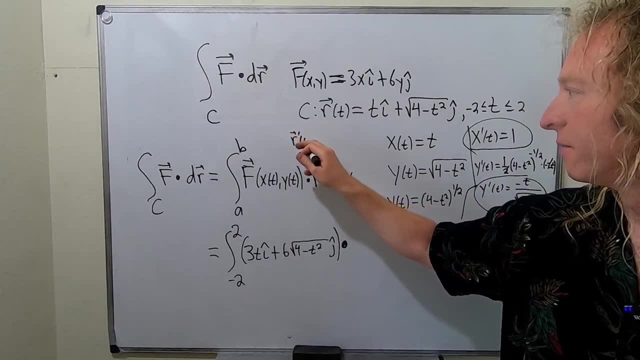 kind like out the numerator either way. and then let's have the Newton depois d손, the derivative of this. so we can kind, we can kind kind get to thatkef, get to that, so we can kind of- I mean, I could write it here- the derivative of this would simply be: well, 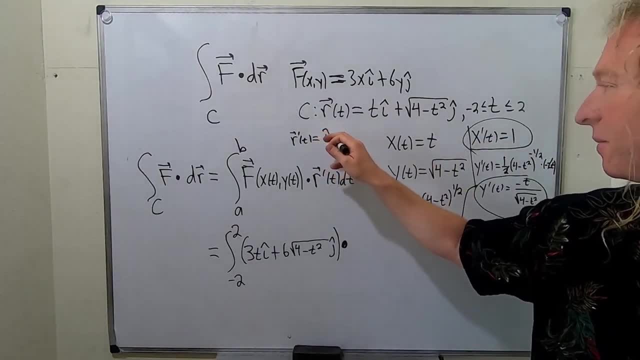 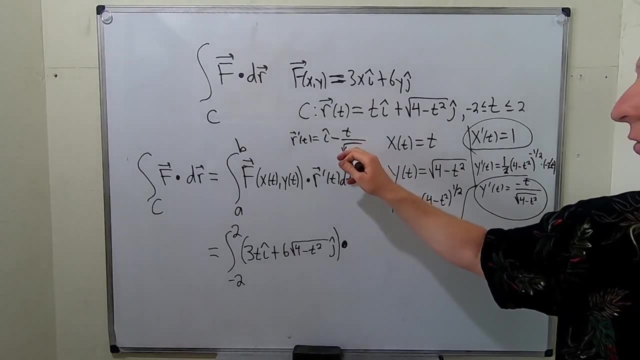 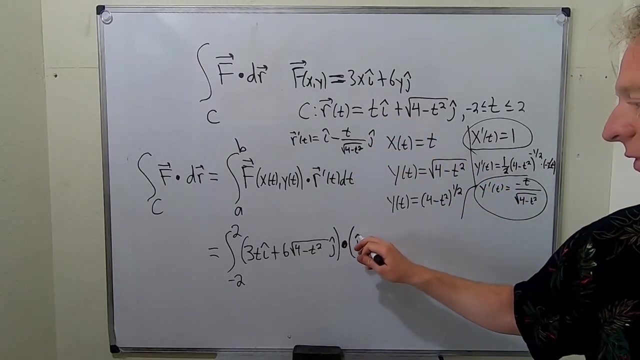 the derivative of that is 1, so just be I hat, and then minus T over, and then this square root 4 minus T, squared J hat. so I'm just going to write this down here now. so it would be I hat minus, and then Y prime would be this piece here. so kind ofружi, bawak ang the derivative in a square root. square root four minus tw al and it's going to go take four at 3 times 2.. I fatty, So you know, I tapped my ENDS읒 and I took my. 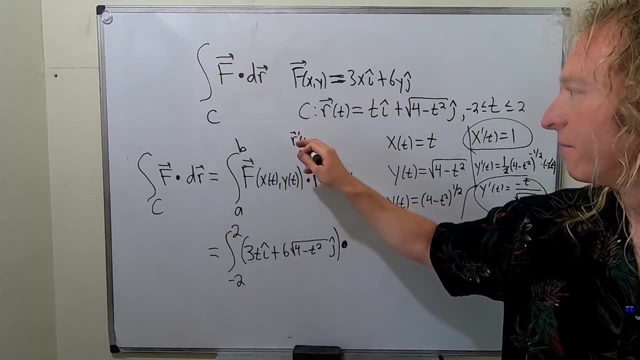 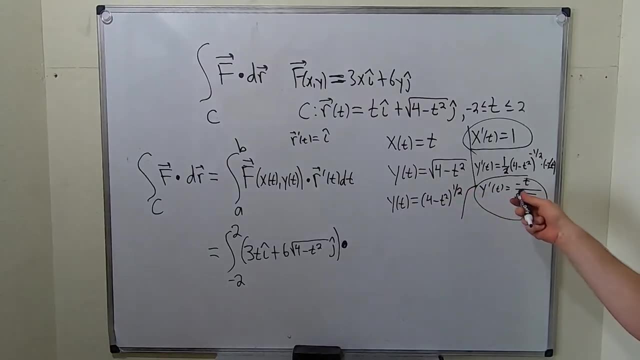 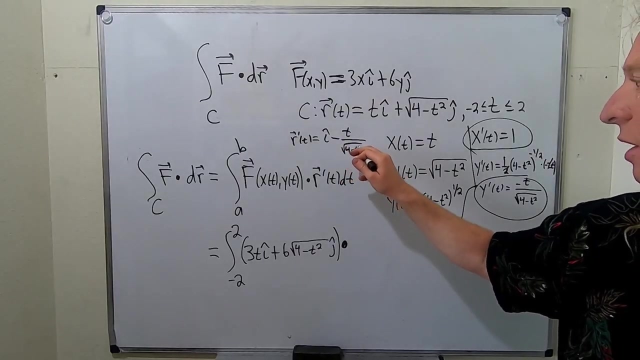 of. I mean, I could write it here. the derivative of this would simply be: well, the derivative of that is 1, so just be I hat, and then minus T over, and then this square root, 4 minus T, squared J hat. so I'm just going to write this down here. 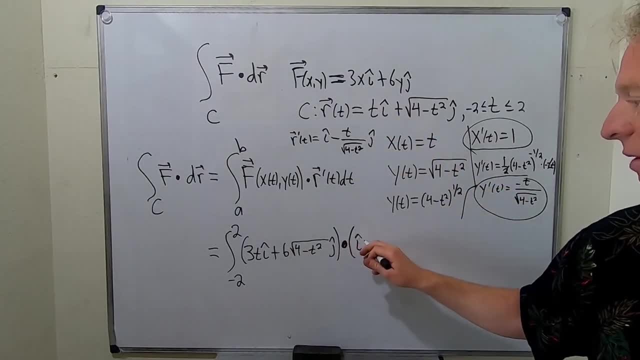 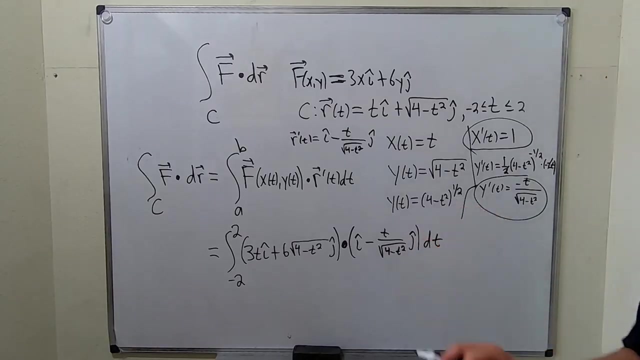 now. so it would be I hat minus, and then Y prime would be this piece here. so minus T over square root 4, minus T squared, and then we have the J hat and then don't forget the DT. so it's really funky looking. I think it helps when you 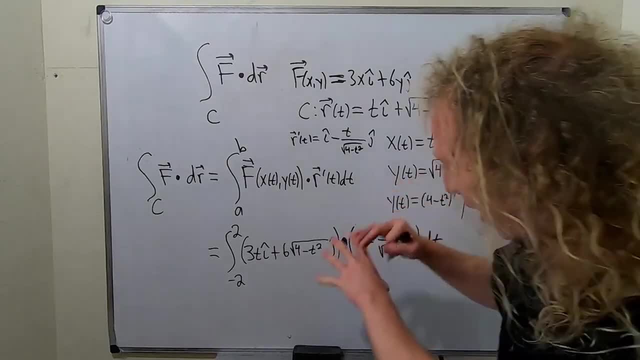 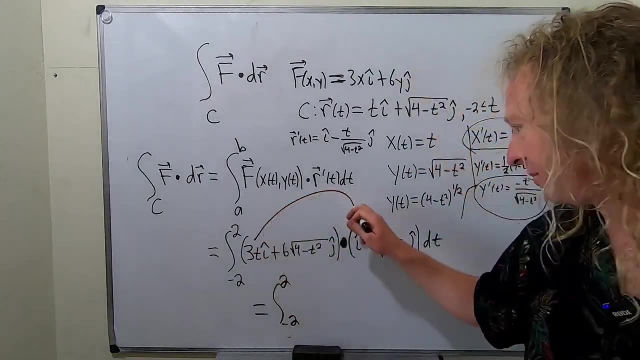 make a dot really big. it just makes it easier to look as a big dot product. so this is equal to negative 2 to 2. so we take the dot product. so it'd be this times this: you don't multiply the- I's right. the dot product is a scalar, so the 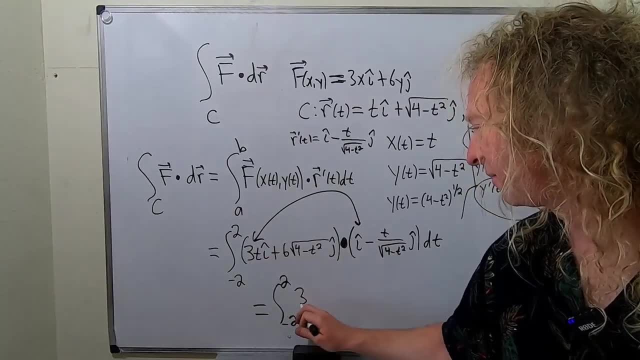 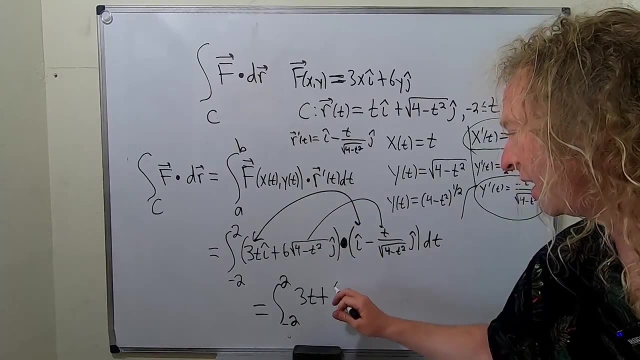 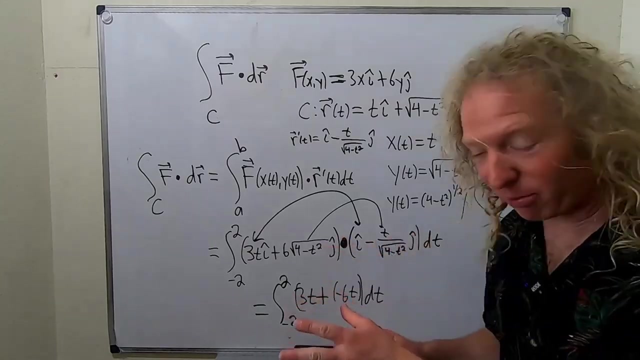 vector goes away now. so 3T times 1 is simply 3T, so plus. and then this times this, so these beautiful square roots cancel. so you just get negative 6T DT, right, beautiful, it just all went away because it's the dot product, right you? you multiply this times 1, so 3T times 1 is 3T, then you. 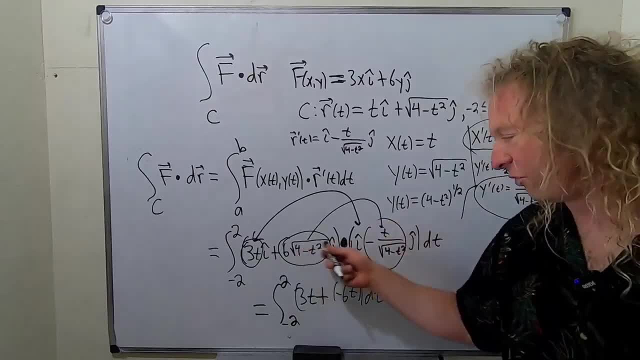 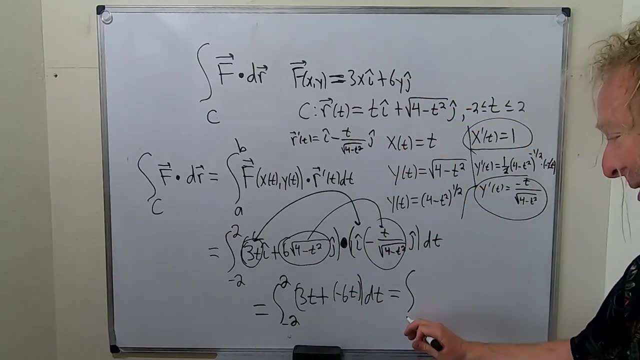 multiply this times this so the square roots go away, so you just get negative 60. it works out really nice. like how do you go from all of this to this? it's just the problems for definitions and we're going from 2 to there. we have picture. 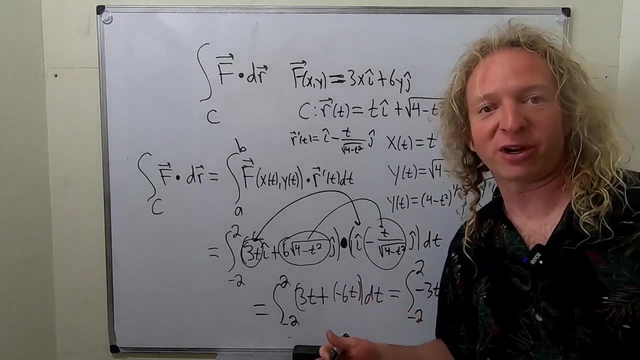 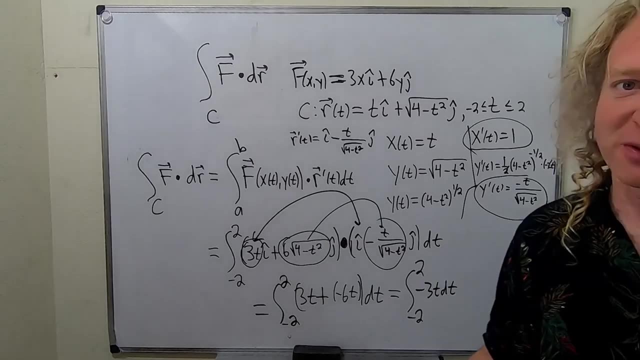 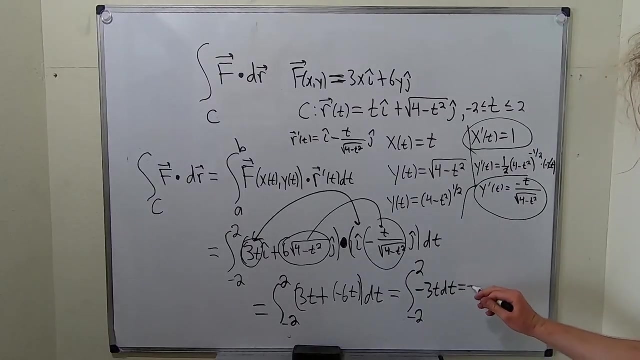 so this is negative. 2 to 2 negative. 3 TM X Trudy column, problem on NG's. so this is negative. 2 to 2 negative. 3 T Mineodi column above that, which represent out all the elements of them. yes, correctly, so we get investigators. 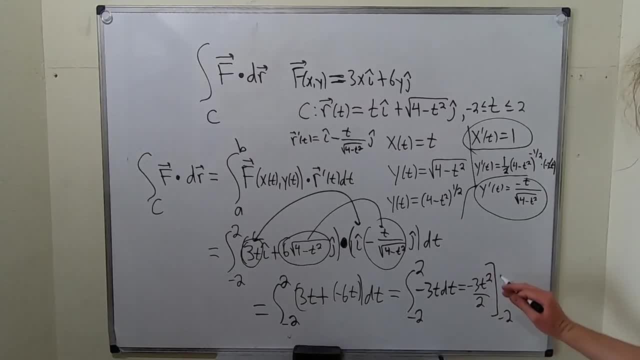 and now that that's explained, you're going to need to Judaism. that's going to do it back, so that your expression, your expression of them, is right now. above all, that's going to get you everything that's you've gotten. so this is a little bit. 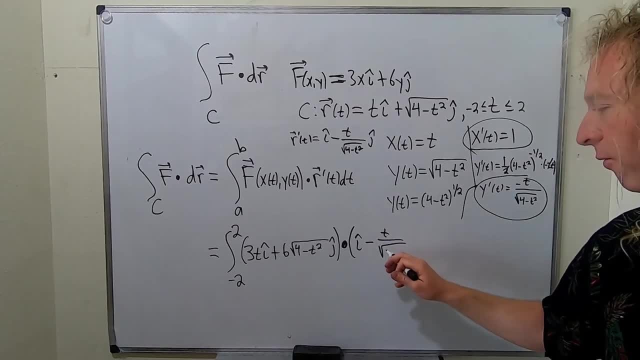 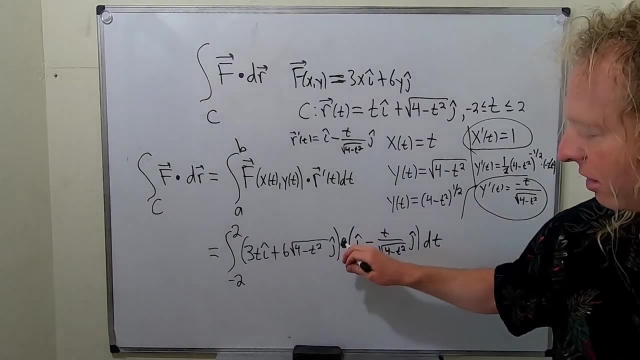 minus T over square root, 4 minus T squared, and then we have the J hat and then don't forget the DT. so it's really funky looking. I think it helps when you make a dot really big. it just makes it easier to look as a big dot product. so 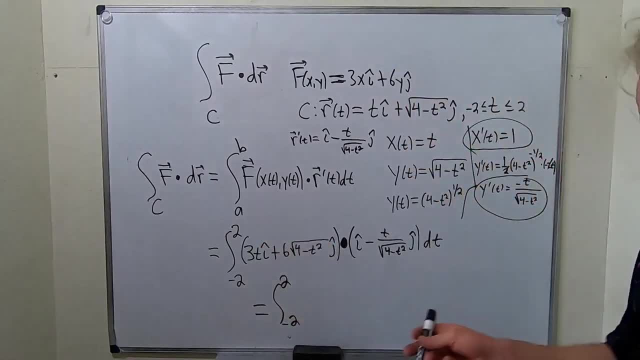 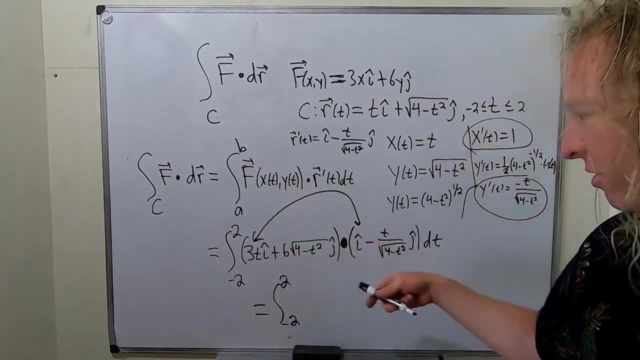 this is equal to negative 2 to 2. so we take the dot product. so it'd be this times this: you don't multiply the I's right. the dot product is a scalar, so the vector goes away now. so 3T times 1 is simply 3T. 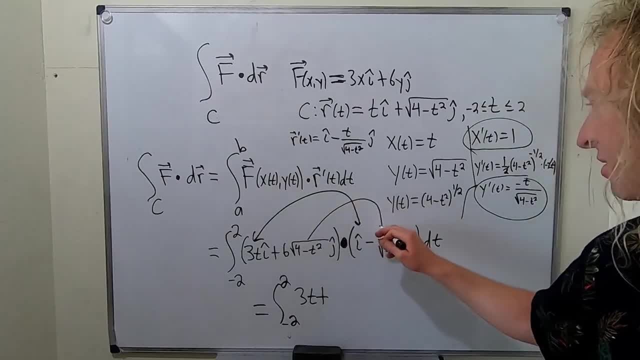 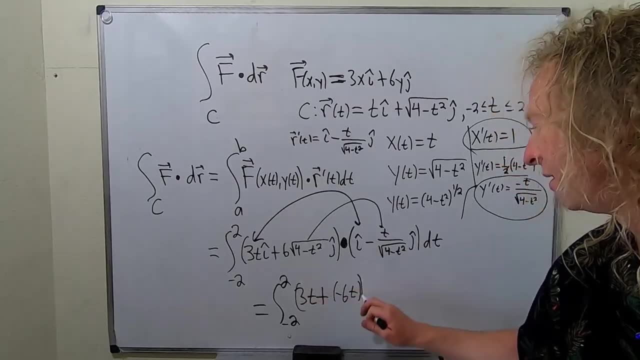 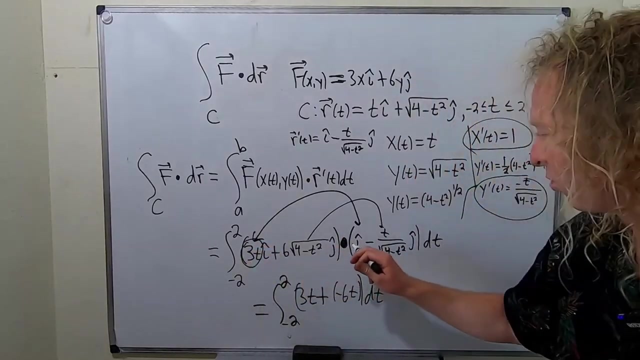 so plus, and then this times this, so these beautiful square roots cancel, so we just get negative 6T. DT. right, beautiful, it just all went away because it's the dot product, right you? you multiply this times 1, so 3T times 1 is 3T, then you: 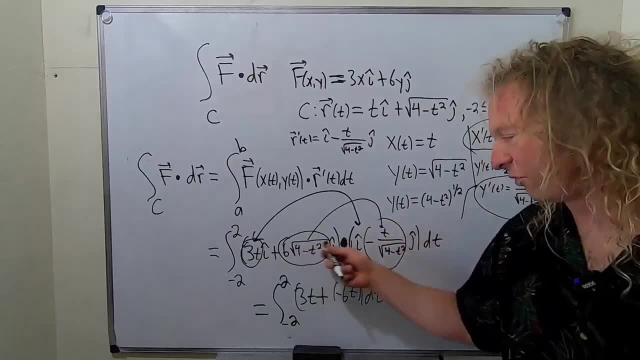 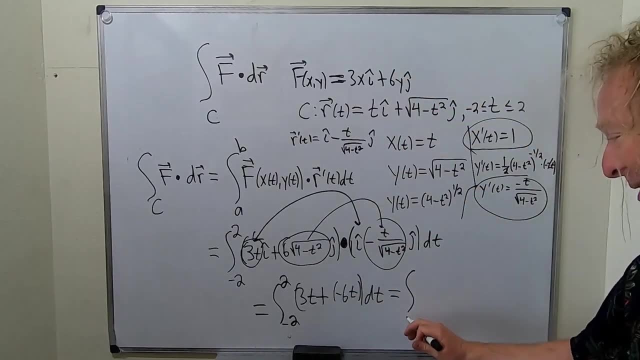 multiply this times this so the square roots go away, so you just get negative 60. it works out really nice. like how do you go from all of this to this? it's just the regular Mach numerator are said, so this is negative 2 to 2. negative 3T DT. 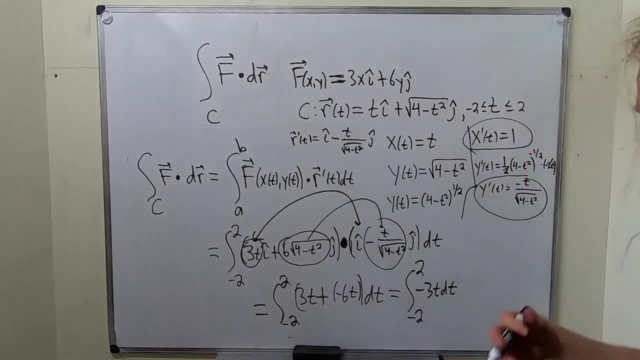 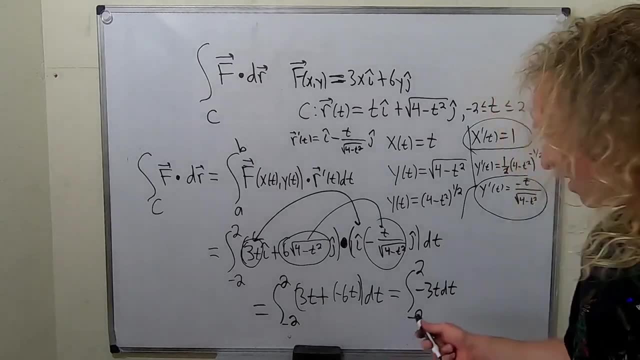 and again. this is something it's used to compute work in physics. it's really a physics thing. I mean it's math, but physics people use this a lot. there's a couple ways to do this. method 1: realize this is an odd function over a symmetric interval. so the answer is 0. 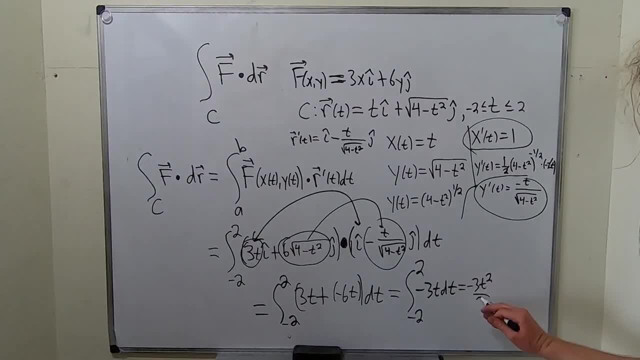 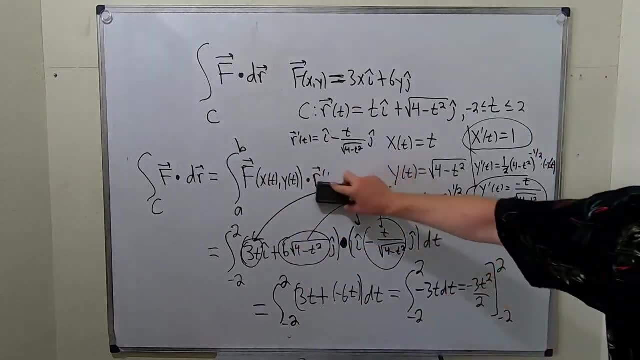 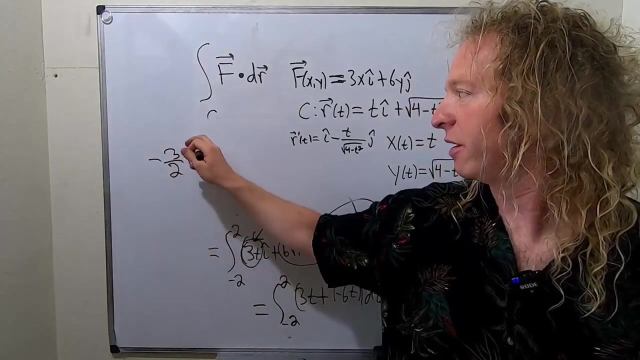 method 2, just work it out. this is negative 3T squared over 2 and we're going from negative 2 to 2. ok, let's finish. I'm going to erase this up here and can continue. erase this, So we have. I'm going to write it again over here: negative 3 halves t squared. 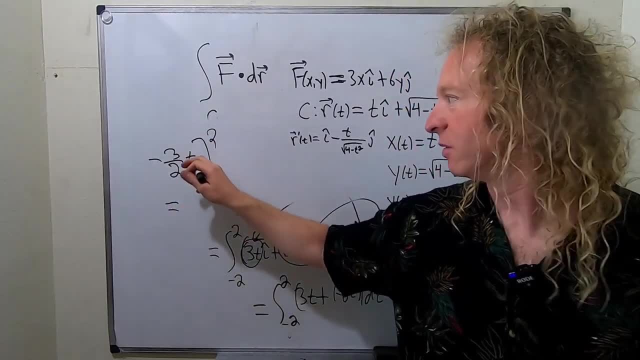 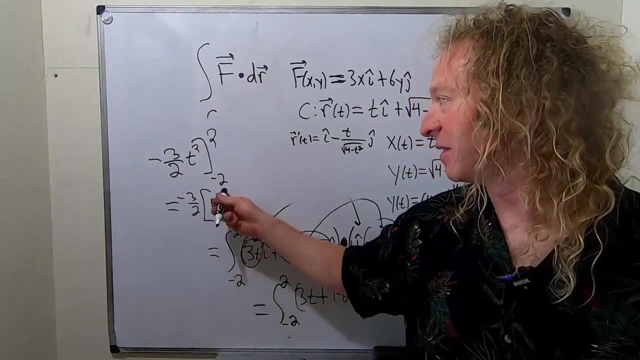 negative 2 to 2.. So you first plug in the 2. Whoops. So you get negative 3 halves. I'm going to mess up now. That'd be bad. 2 squared is 4 minus and then negative 2 squared is also 4.. So you get. 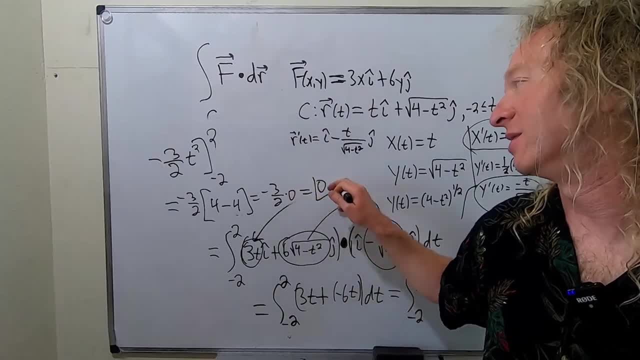 negative 3 halves times 0. So you get 0. And that is the final answer. I hope this video has been helpful. Take care.